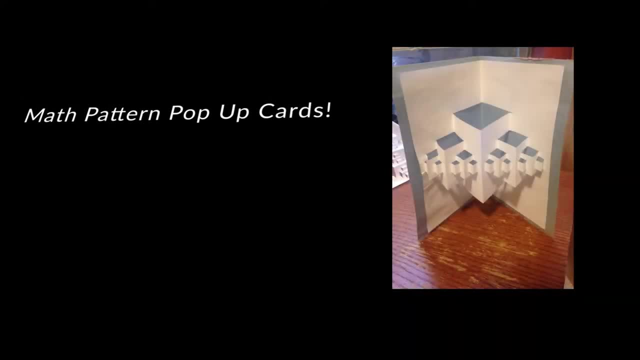 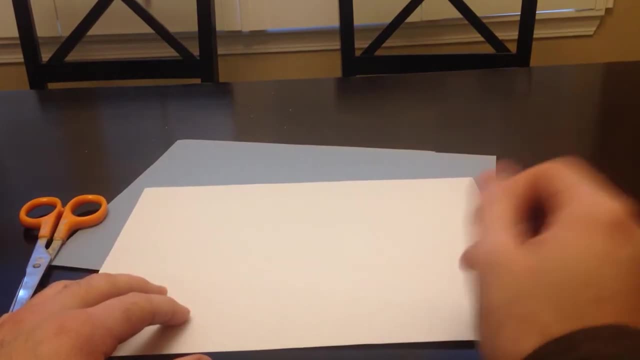 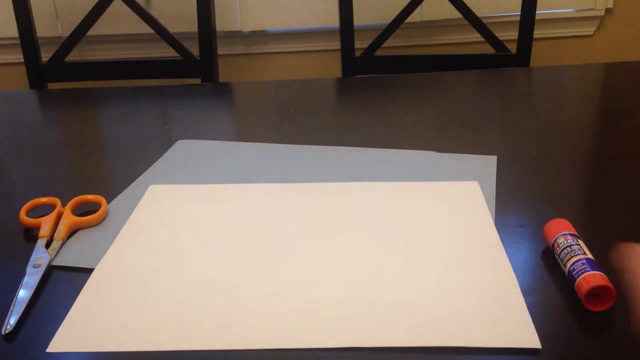 All right, so here are the directions for making this kind of fun holiday little mathematical surprise treat. You can hang it on your fridge or whatever you want to do. Okay, so the necessary materials is definitely a piece of paper, definitely a pair of scissors. 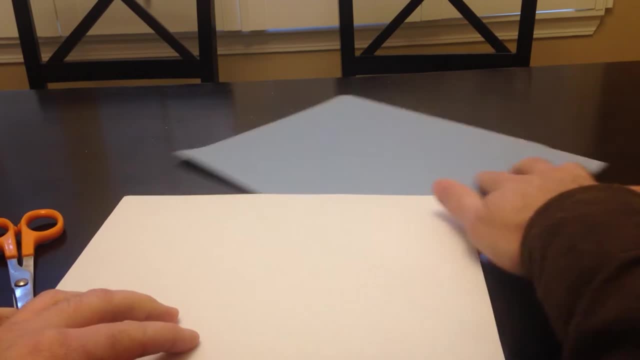 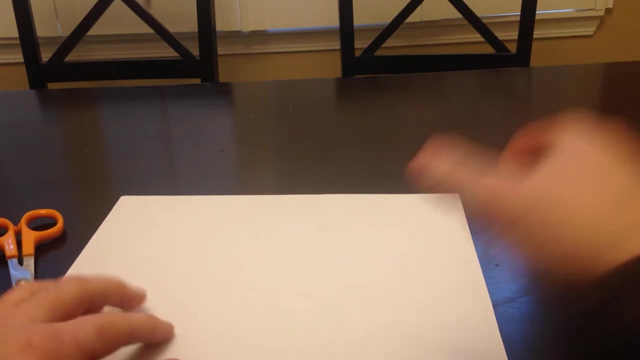 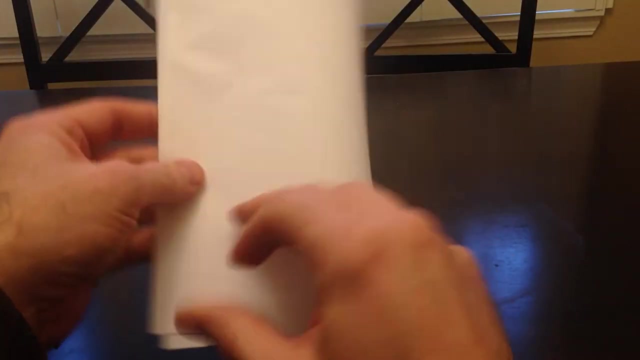 If you want, you can have a glue stick and a construction paper of your choice at the very end. We'll see when we do that. Okay, but first take your piece of paper, fold it along. What do they call that? A hamburger fold. 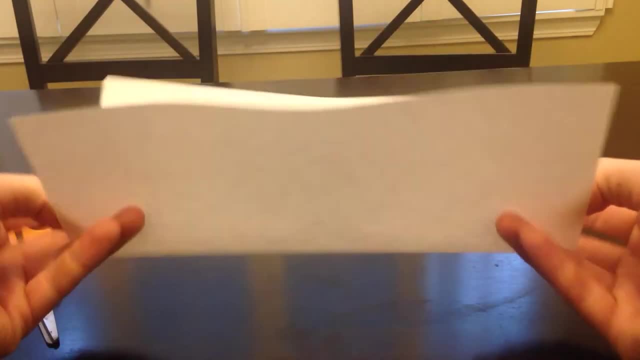 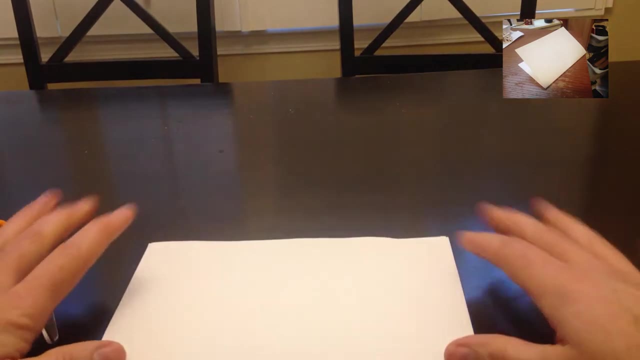 Okay, you don't want to make the narrow one, Don't do it the narrow way. Do it the long, the other way. Okay, line it up, Give yourself a nice crease, Okay, so you've got a V, just like that. 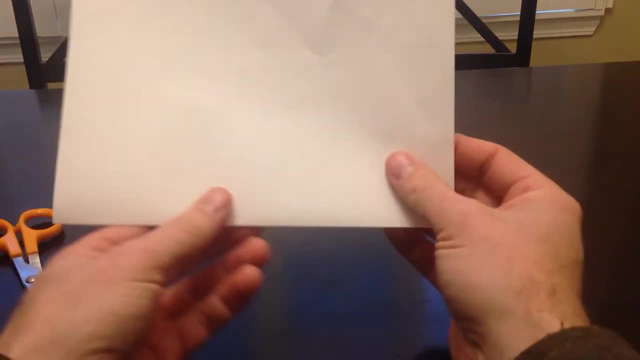 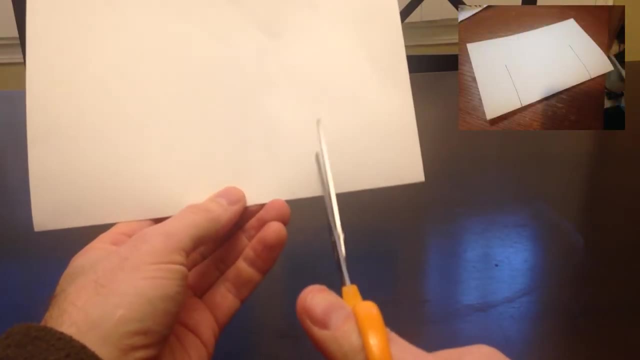 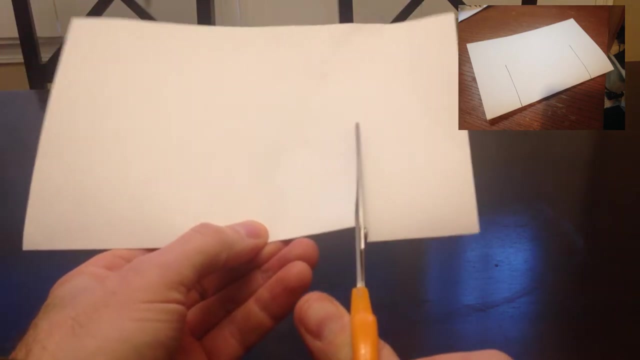 Okay, with the fold at the bottom, we're going to be making two cuts. Make sure you plan first before you cut. and it's going to be, and it doesn't have to be exact- it's about one quarter of the distance across and we are going to cut straight halfway. 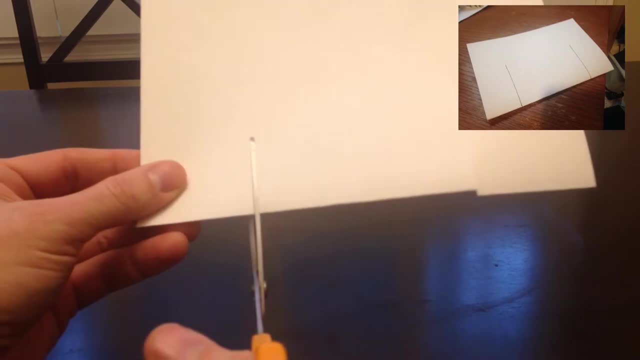 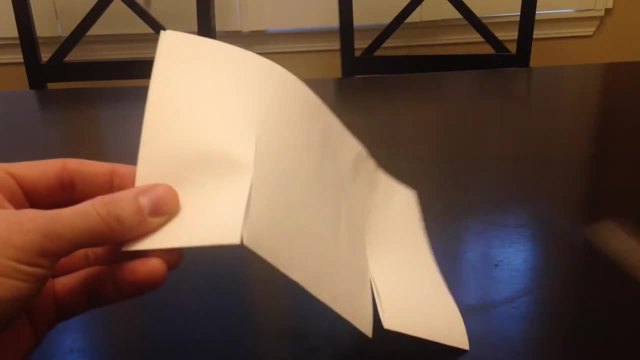 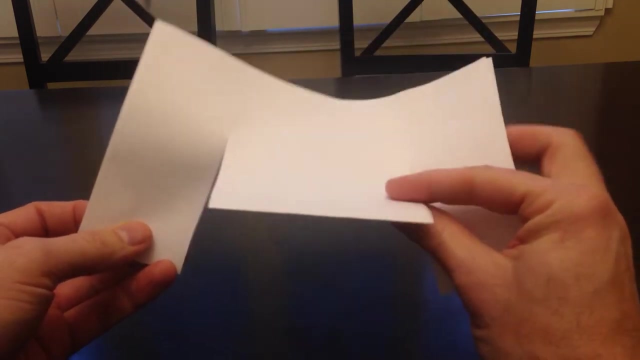 You're going to do that on the other side as well, About a quarter of the distance across, halfway up. That is your first cutting. Okay, look at that. So you're going to take this middle flippy flap and you're going to fold this up. 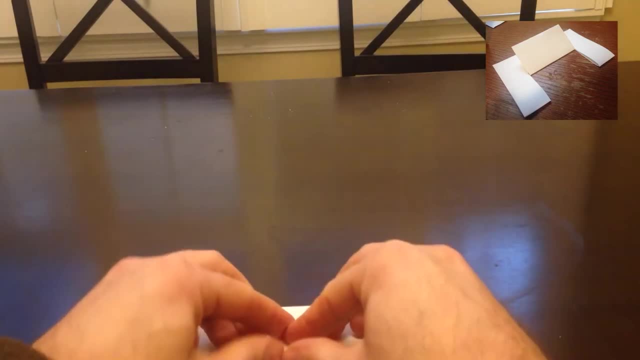 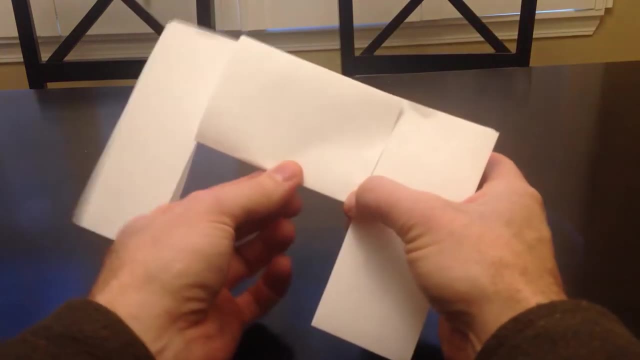 You fold it so it goes all the way to the very tippy top. You fold it up so it goes up to the top And make a nice crease. Okay, you will fold it around the back side and fold it just to the top. 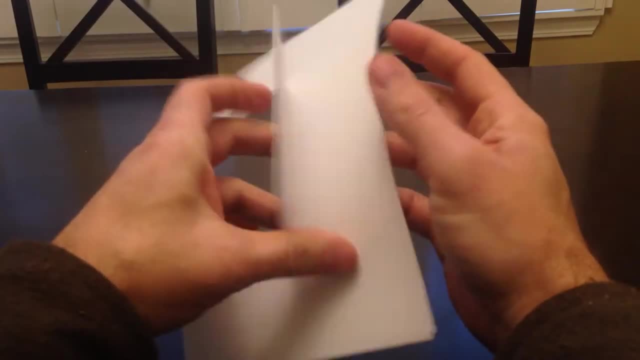 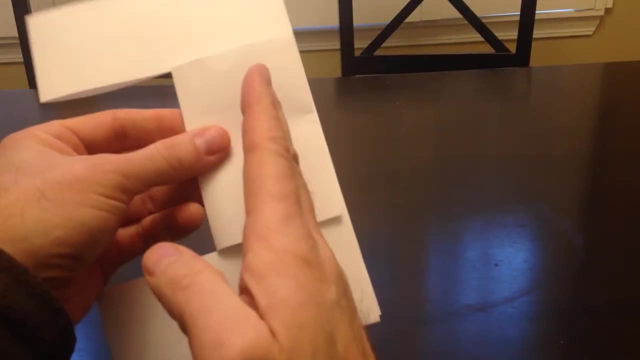 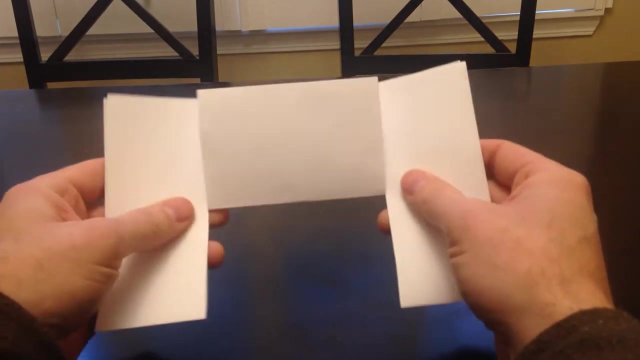 Okay, notice that when I cut mine, I cut mine a little bit too far right there, but I only folded it to the top. I didn't fold it past and I didn't fold it before. Okay, so if you need to cut it a little bit more, do so so it can reach all the way up to the top. 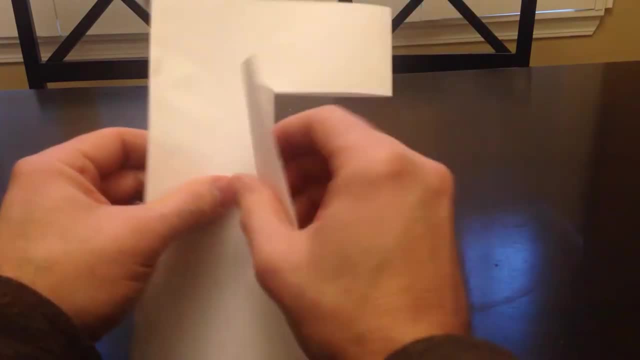 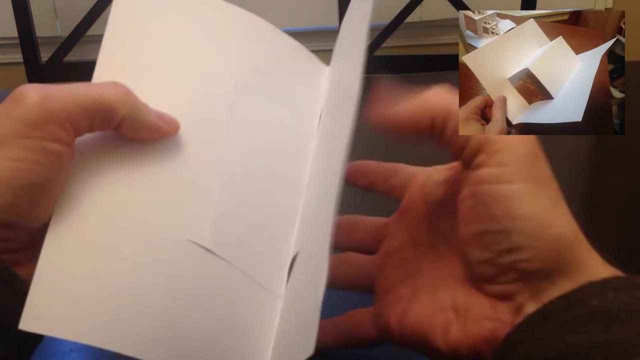 Okay, here comes the fun part. This is the pop step. Okay, bring that flappy flap down and then you open it up a little bit. You're going to take just the middle part and you're going to turn it inside out. 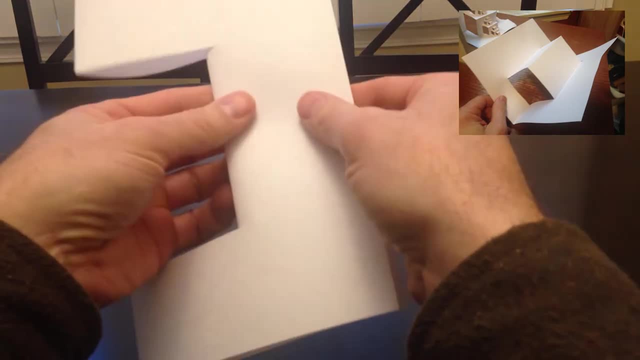 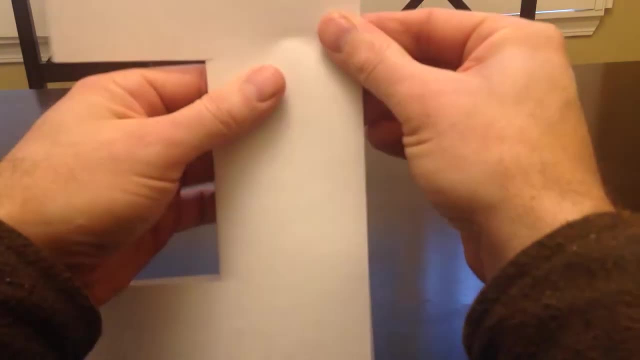 Look at that And then so it's turned inside out and then you smoosh it shut. So you've smooshed it shut inside. Do your best to keep it lined up, but it doesn't have to be perfect, Okay. 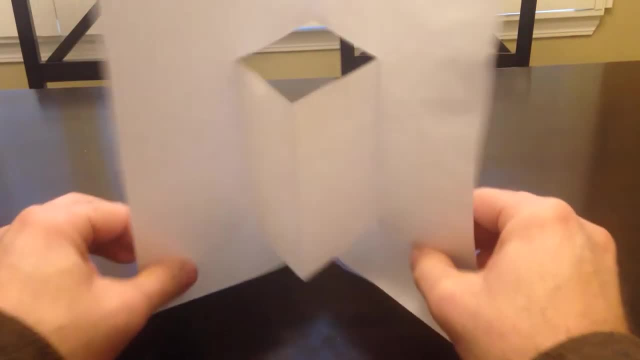 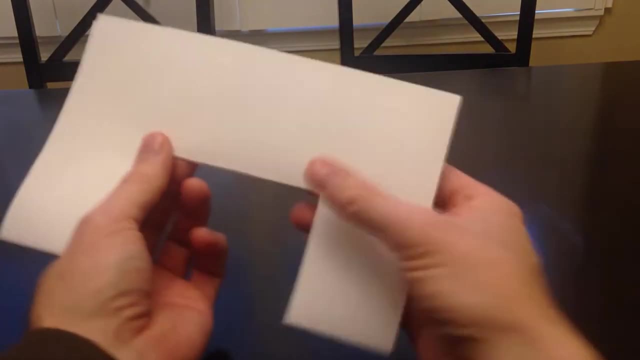 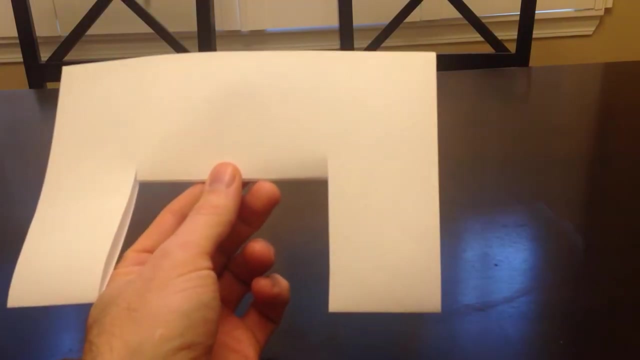 Okay, Look at that Fun shape. You could call that a day, but we're going to go on. We're going to continue this what's called a fractal pattern. Make sure everything is tucked up inside. We're going to do it again the same thing, except we're using just this middle segment here as our guide. 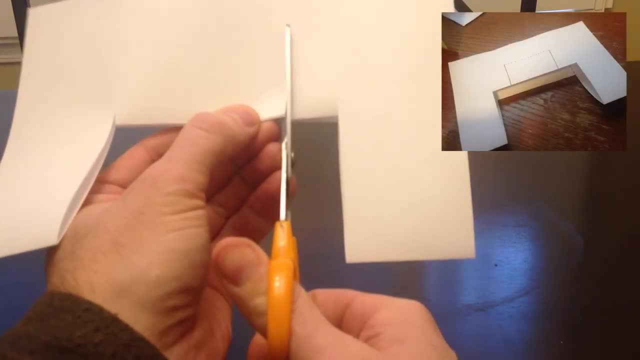 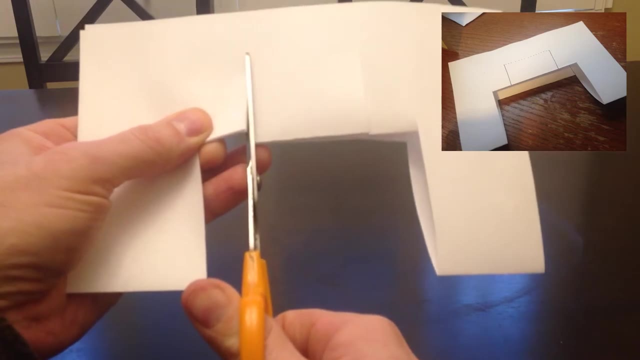 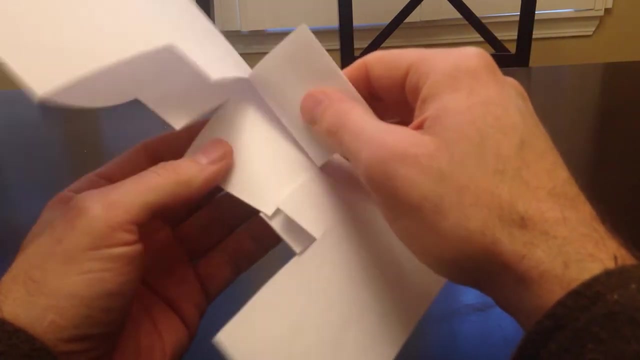 We're going to go about a quarter of the way across, Cut halfway to the top. Same thing on the other side: Quarter of the way across, Halfway up. Take the same flap. now There's going to be two pieces, so be careful. 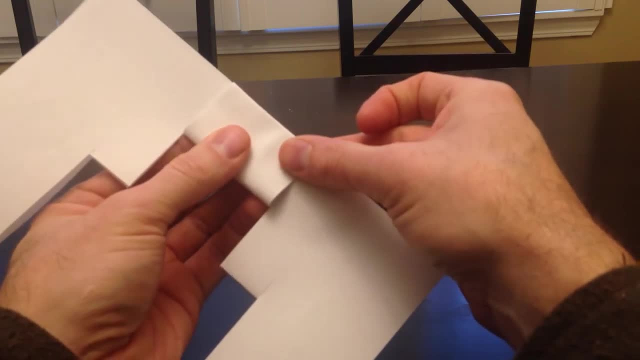 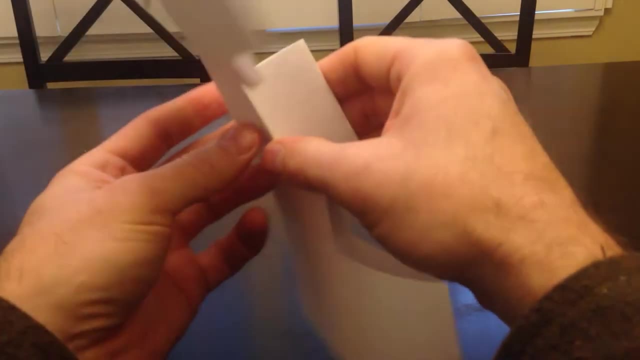 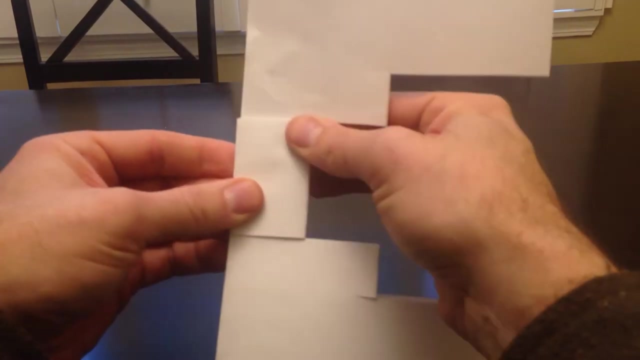 Grab them both, Fold that up to the top And crease. Okay, just to make it work better, you take that same section and you flip it around to the other side, Fold it, Crease it, Bring it down. 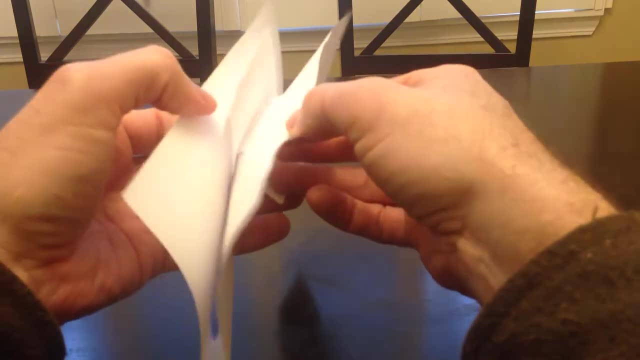 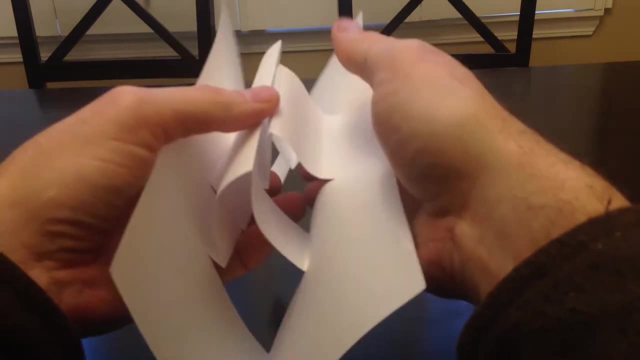 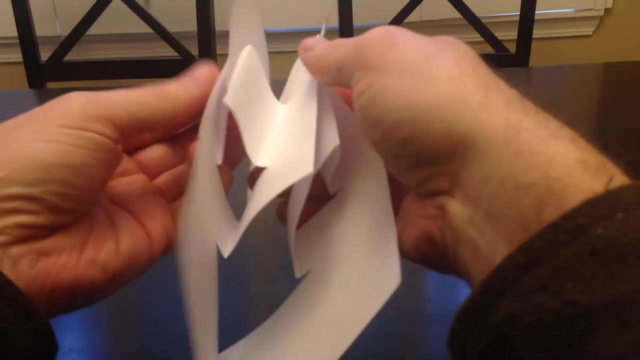 Open it up a little bit And you're going to take those flippy flaps- we just did and you're going to pop them up, Push it from the underside, Push it up So it goes up there and then close it. 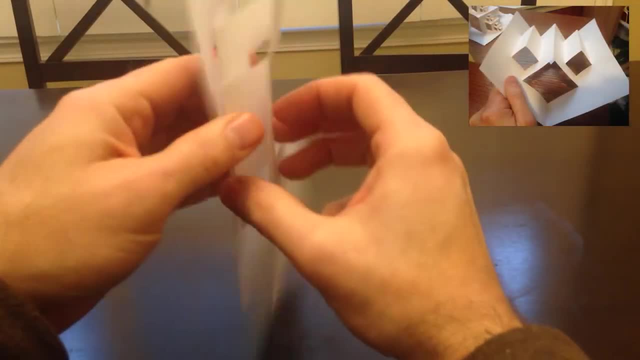 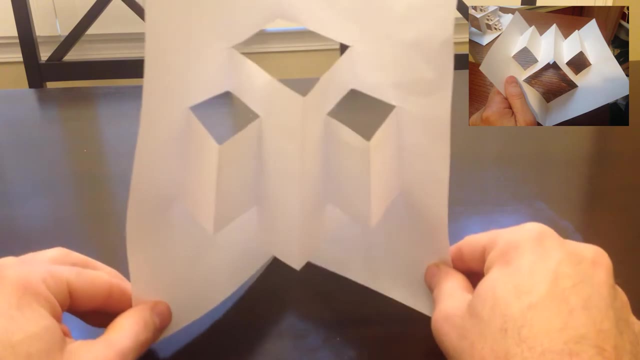 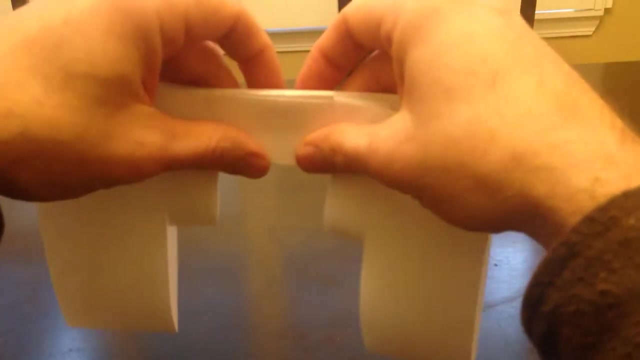 Crease it nice, Open it up to see what you've created. Look at that. It's a repeating fractal pattern. Okay, how about that? We're going to do it again, just because Do it as many times as you can with a good, sharp pair of scissors and nice folds and clean folds. 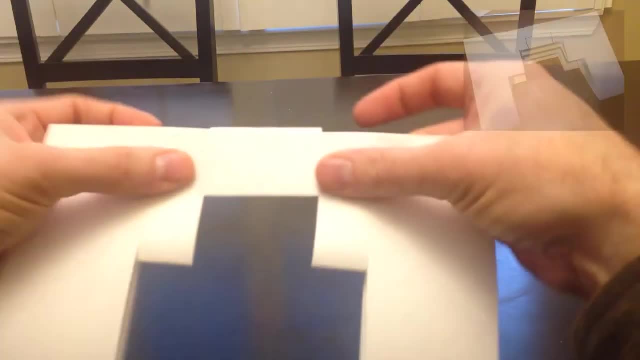 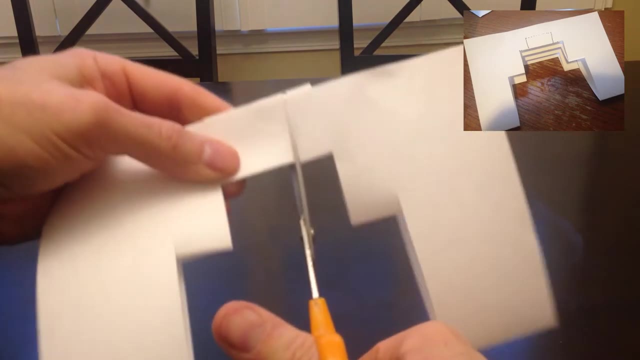 So we've got everything tucked up, folded up. There you go Quarter of the way across. Again halfway up. It's getting smaller but notice it's getting harder to cut. It's because you're cutting through more folds of paper. 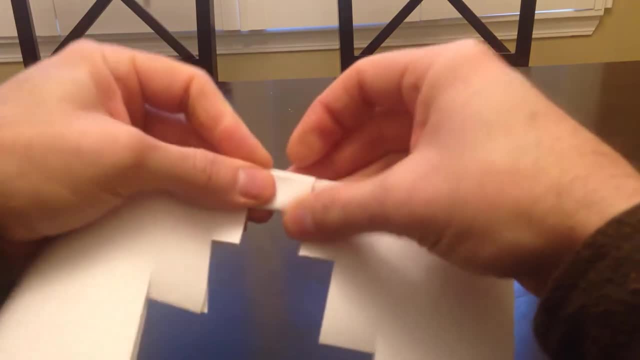 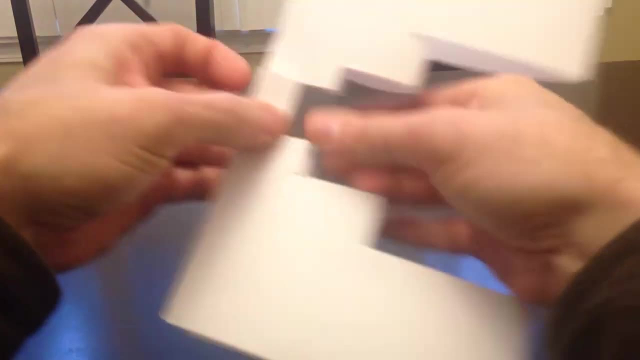 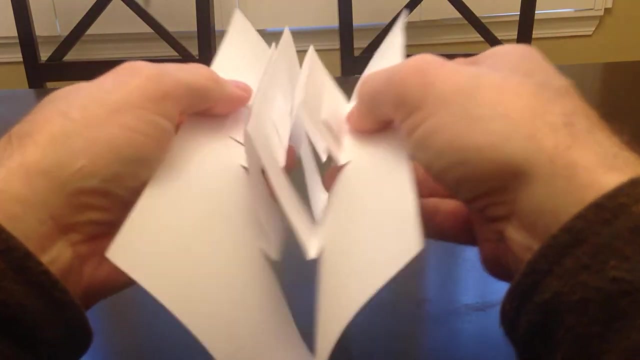 Okay, so you take those. You take those little folds, you just did. Fold it up to the top. Repeat those steps. Okay, All right, Back and forth. Creasing it, nice, Open it. We're just repeating every single thing we've done. 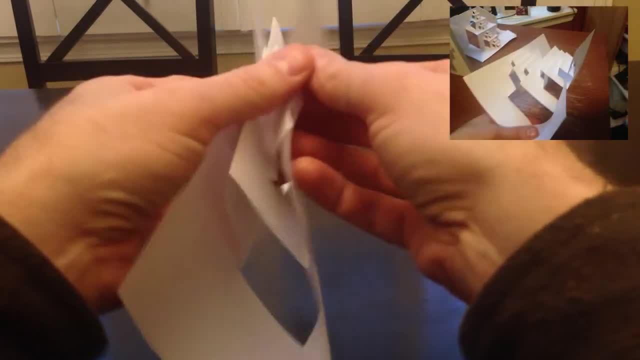 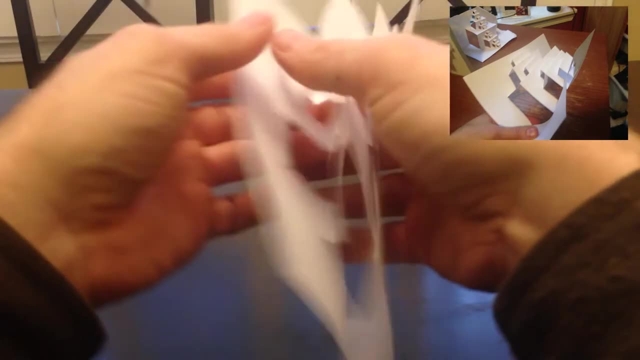 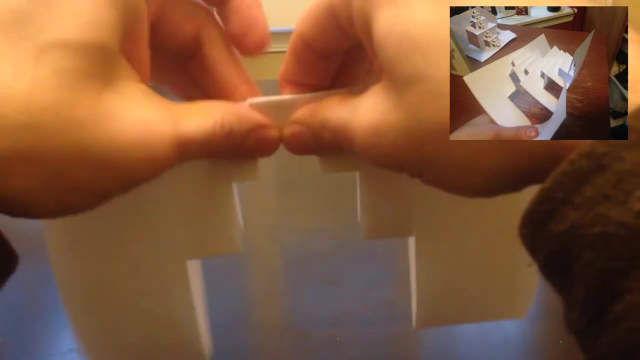 There's just more this time. Pop them each up, Pop up, Open a little. Pop it Up, Open it, Pop it. Hey, They're a little tricky. as you go further on, Close it all back, Okay. 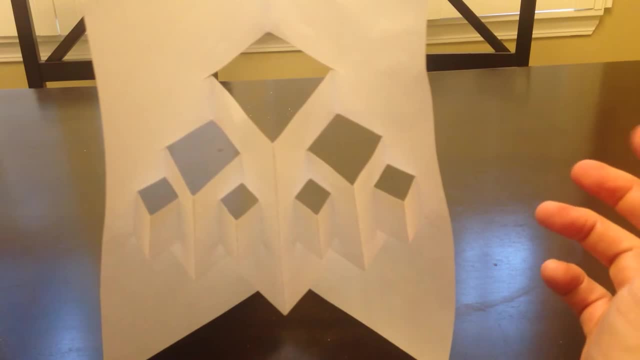 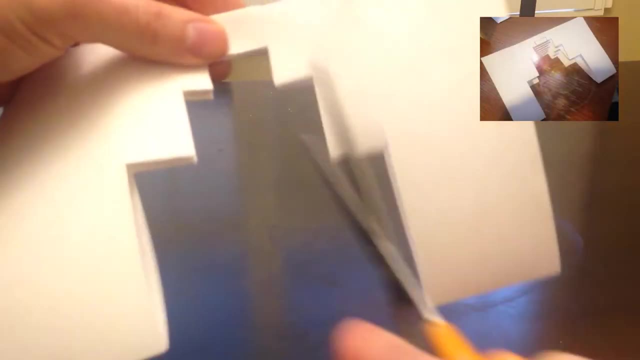 So look at that. Super nice. I'm going to go one more level, but you can call it quits with this Quarter of the way, in halfway up. Be careful, you don't want to cut all the way through If you do. 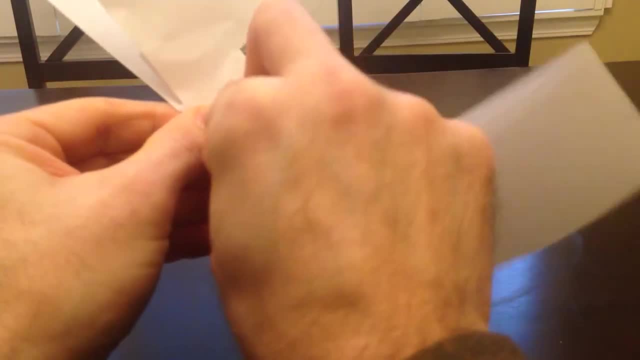 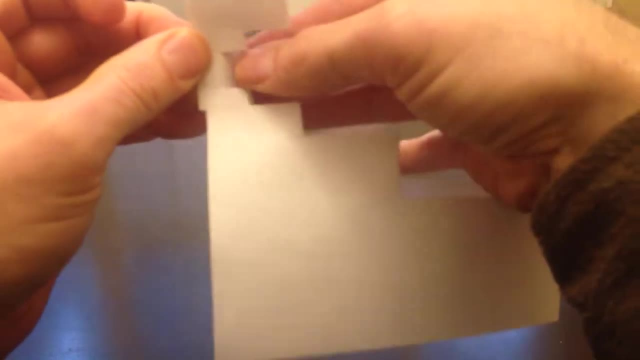 it's going to look like your bottom. It's over. It looks pretty, but it's no longer the same thing. There's a whole bunch of them this time, so fold them all up one way, Fold them the other and crease. 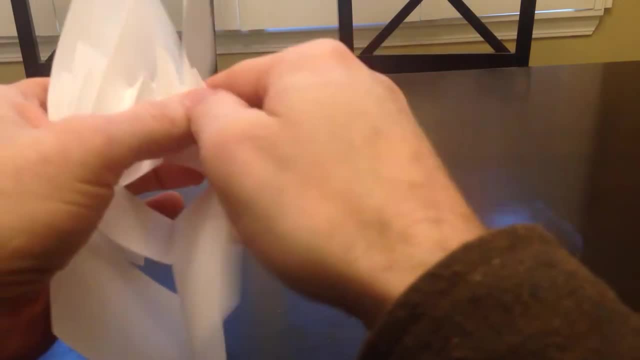 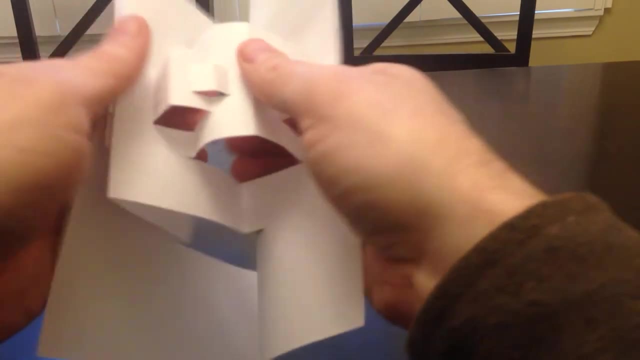 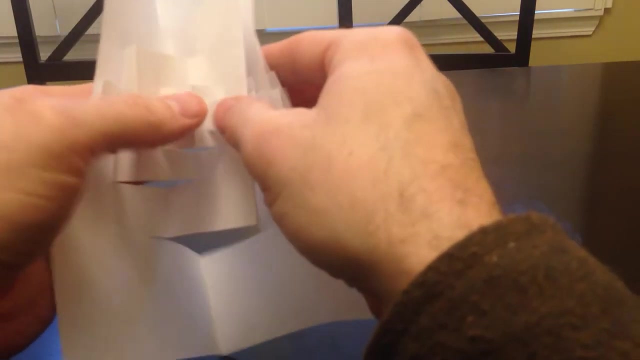 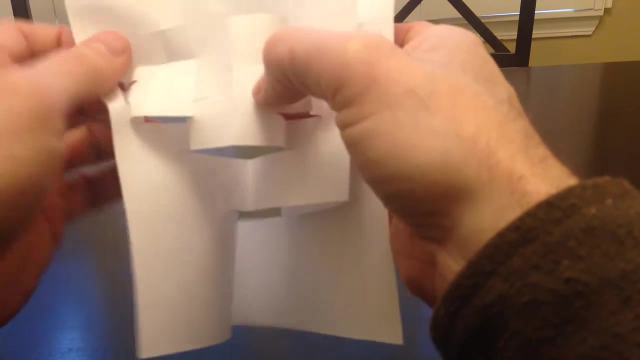 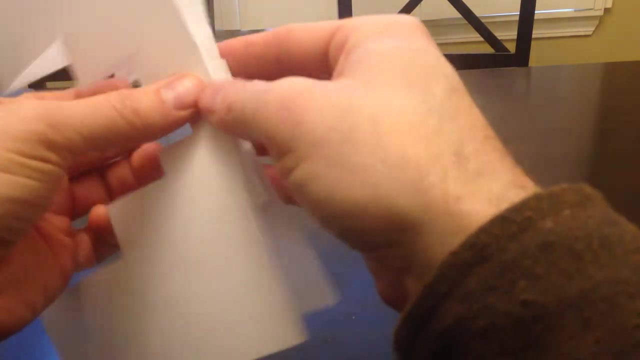 Open it and then pop, Pop each of the little pieces in. That's my favorite part, right there. So if anything gets pushed down, you have to re-pop it all up. It takes a little bit of time, Just be patient. Once you've got them all popped up, squeeze it shut. 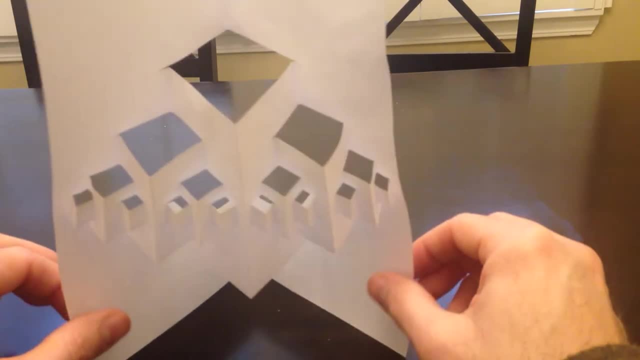 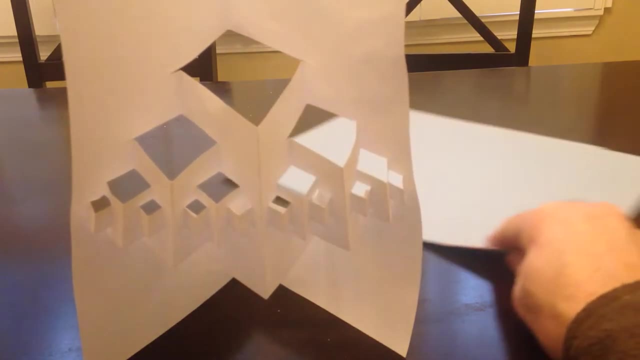 And then what? That looks incredible. Okay, for the final touch. you can go further, but I don't recommend it Because you might cut all the way through. To make it a nice backing, take a piece of construction paper, any color you want. 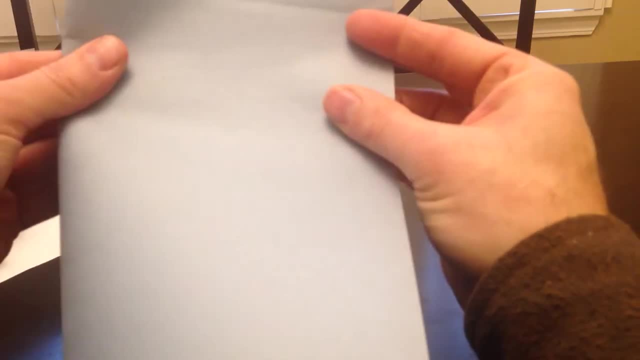 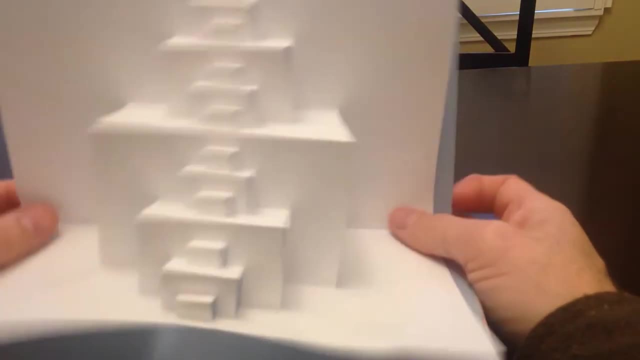 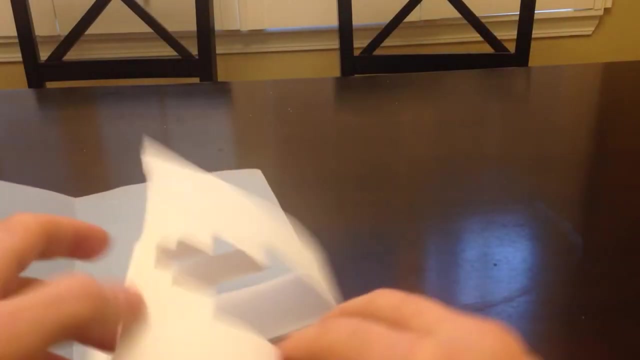 Fold it the same way, Nice. What's going to happen is you're going to glue this piece into it, So you're going to make a nice little card. So to get it to glue right, smush your creation, Take some glue.